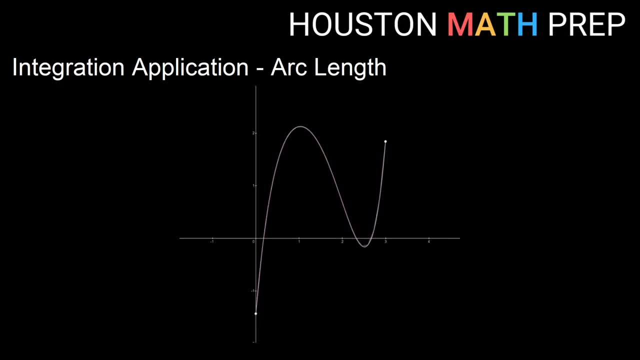 that the approximation that we're getting becomes better and better. We get a more accurate approximation the more subintervals we use. The idea, of course, with integration is that if I can break this subinterval up into an infinite number, or approaching an infinite number of 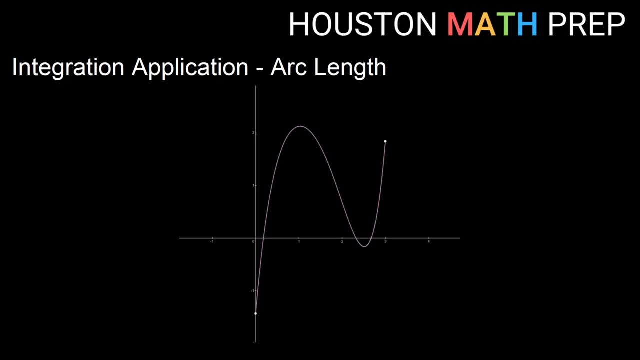 subintervals and then add those distances together. we will use an integral to do that and we'll get the exact length around the curve. Let's look at how we might do that. We're going to zoom into one of our little subintervals. 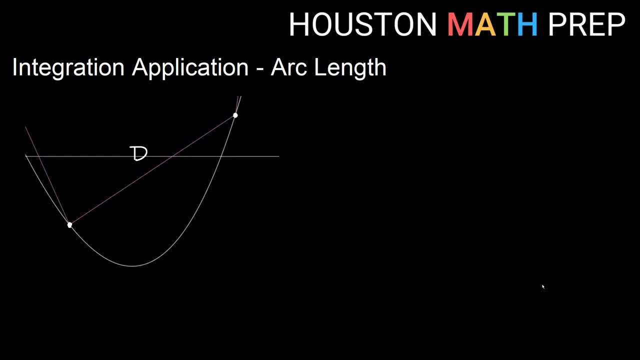 So here, let's say, I've zoomed into one piece of my approximation. Our approximation is going to be made up of these little distances. Here I've called it d. We want to think of our distance d here as the hypotenuse of a right triangle. That allows us to use Pythagorean theorem with a right triangle. 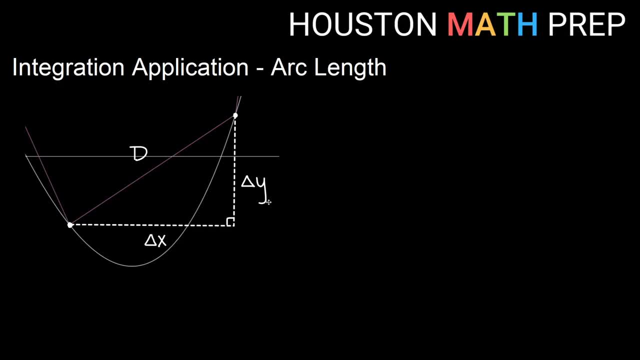 So we have one leg being a change in x- delta x and one leg being distance change in y- delta y, and Pythagorean theorem, distance formula, tells us that if I square these and add them up and then take the square root, that will give us the distance d. Now what we know in calculus is: 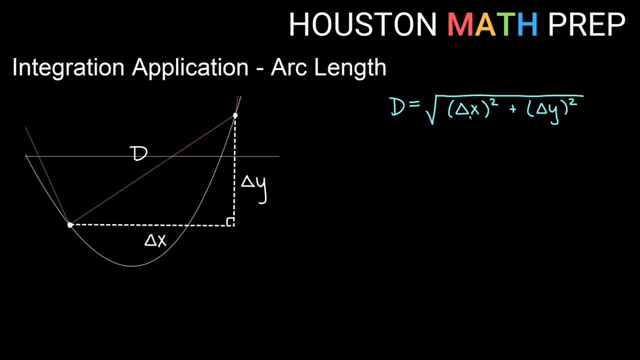 that if we take delta x or we take delta y and we allow those to get smaller and smaller and smaller, they become this idea of dx or dy, this infinitesimal amount of x and y. And so, as we look at many, many subintervals tending toward infinity, then our delta x and our delta. 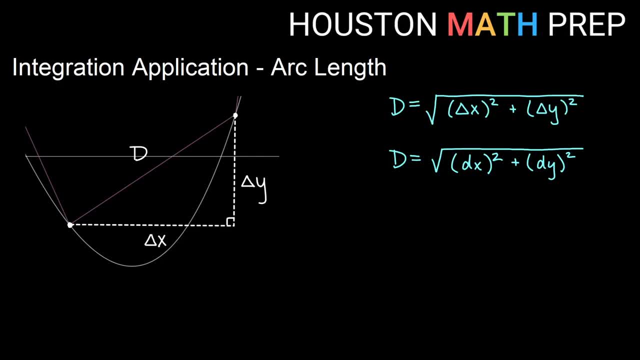 y become these microscopic values, dx and dy- that we're probably familiar with from integration. So the problem with this statement here is that we don't really have anything that I can say. integrate dx, right. So the dx is in here, It's a term, It's being squared, It's square root. We don't really 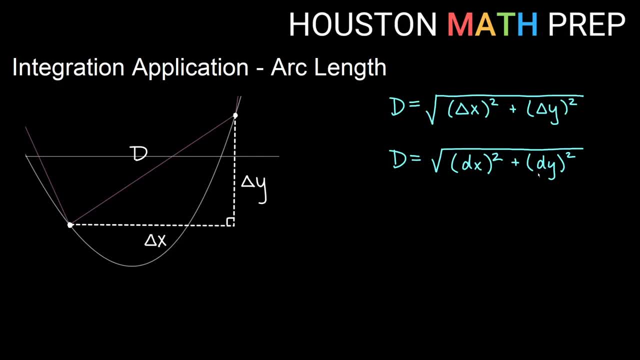 want that. We don't want operations on dx as part of our integral here. So what we really want to do is find a way to get a dx outside of this expression. So what we'll do in here is: we'll have this expression here. This is going to be a square root of x squared plus x squared, So we'll 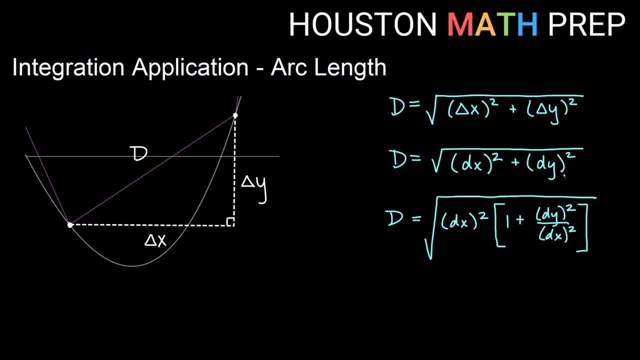 get this expression here. If we factor out a dx squared, there's not really a dx squared in the second term. So when we pull one out, we end up with dy squared over dx squared. So we get this and that dx squared is now sort of separated, And what we'll do with this is we will now pull it. 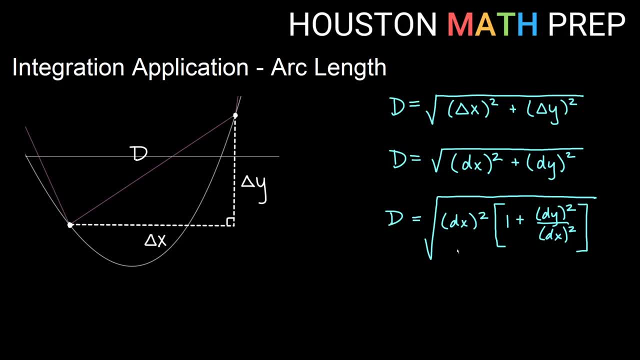 out of the root. It's a perfect square and we can pull it out as a single dx term outside of the root And we will get something that looks like this. So the dx is now on the outside. That looks little more like what we would have in an integral. we have this root, we have one plus and, if I go, 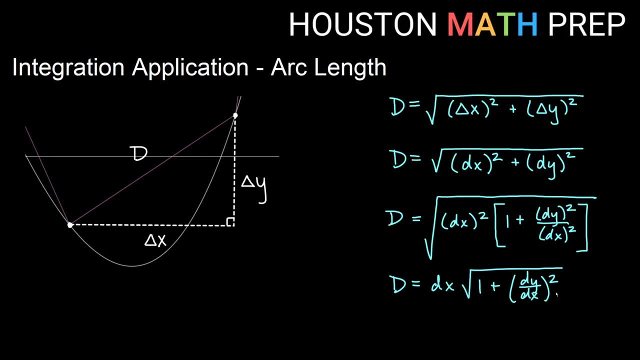 ahead and think of these differentials here as a single fraction squared, we get dy dx squared and this dy- dx we would think of as like an f prime of x, right? so if I bump the dx to the back and I rewrite this in prime notation, then I get this kind of a formula for the length around the. 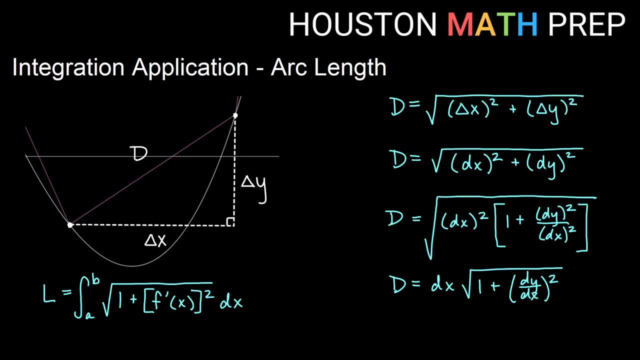 from some x value a to x value b, we get the square root of one plus f prime of x squared. notice that the square only applies to the f prime. so what we would do first is we would find the derivative of f of x. we would then square it, add one to it, square, root it and then 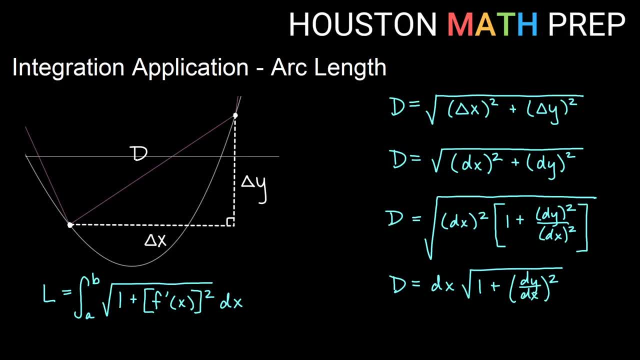 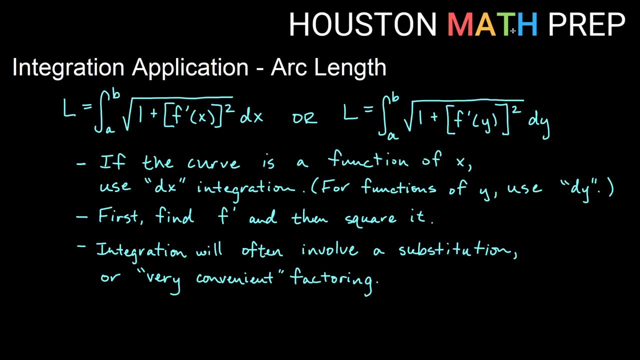 we would integrate it from a to b, assuming that we can do that. so just to wrap up here before you hop along to our example videos, so you can integrate in terms of dy and and and double dx. so just to wrap up here before you hop along to our example videos, so you 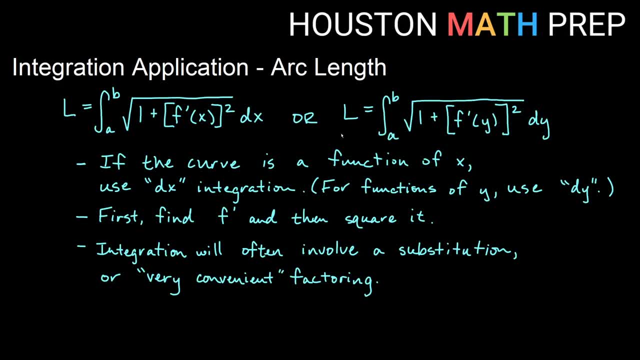 can integrate in terms of dy, dx to x, find y and times y and double dx and then double dx to x and vice versa. dx or dy, depending on if your curve is a function of x or y. If it's a function of x, 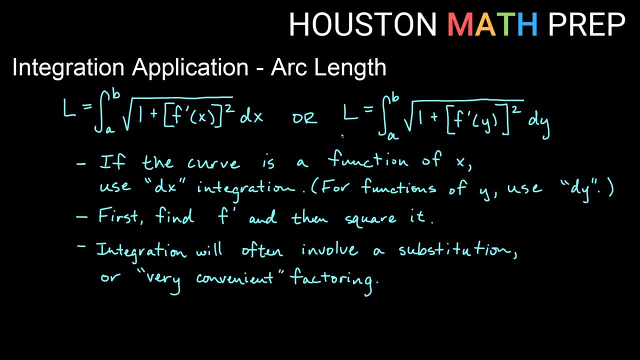 use dx integration For y's, use dy. The first thing you'll do in this process is you'll need to take whatever you have for f of x or f of y and find its derivative. You'll do that and then you'll square it. That will take care of that. Then you'll add one to it and do your. 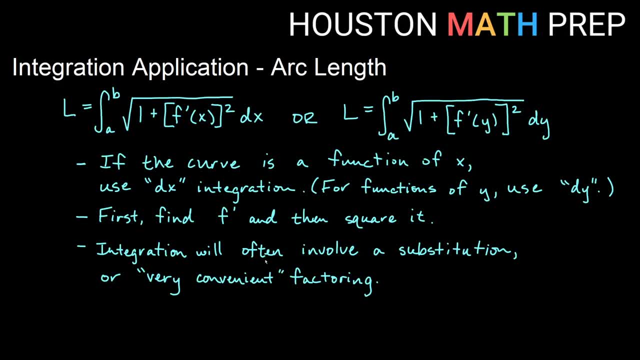 integration. Your integration will often involve a substitution. It's very likely you'll be left with square root of something, or maybe the square root simplifies but you have something sort of odd underneath and maybe you're not sure how to integrate. Oftentimes the integration. 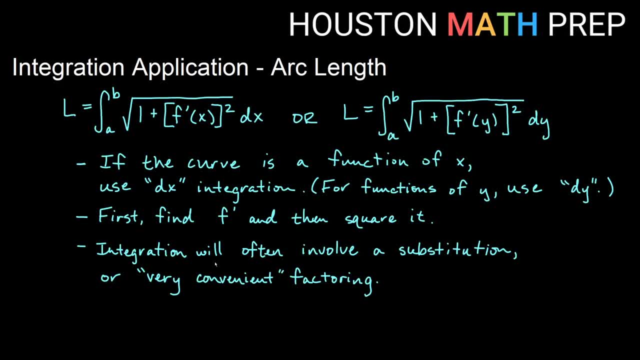 will involve a substitution, or what we're going to call very convenient factoring. Check out our examples- I believe two and three video- You'll see what I mean by very convenient factoring. These problems must have very specific functions to be able to integrate these by hand that you